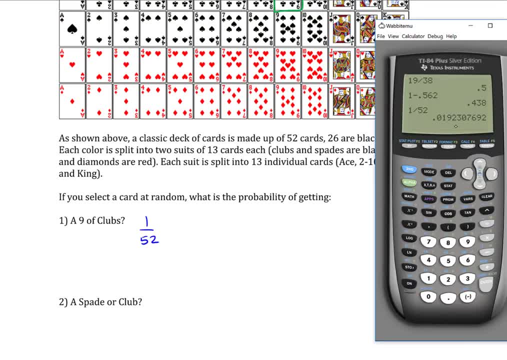 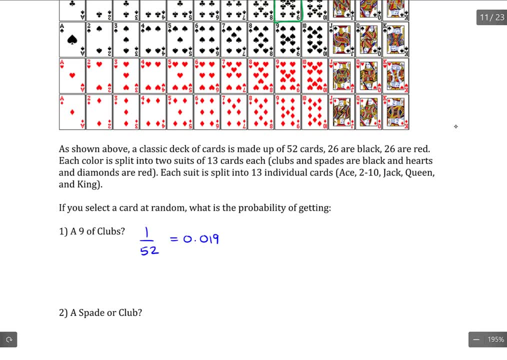 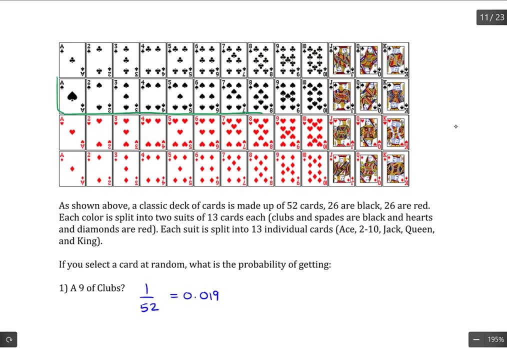 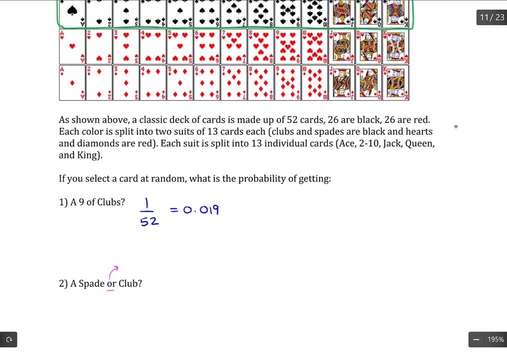 one over fifty two or point zero one, nine, Now a spade or a club. The spades is a suit and it comprises all of these cards, and the clubs is another suit, which comprises all of these cards. The word OR in probability indicates that we need to add these groups. 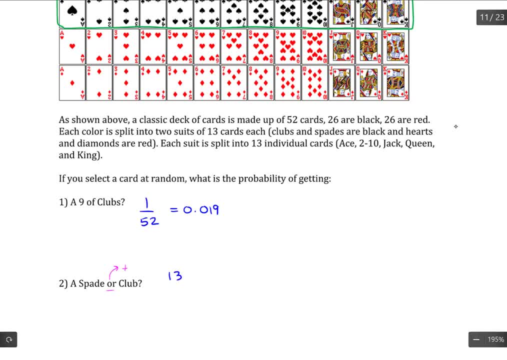 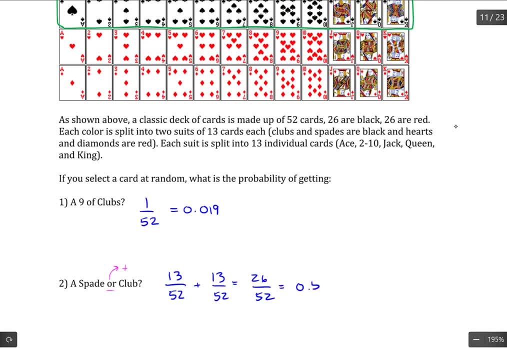 which is 26 over 52, or half of the deck, or 50%. Another way to think of it is: a spade is one of the four clubs, a spade is one of the four suits and clubs is another one of the four suits, So one. 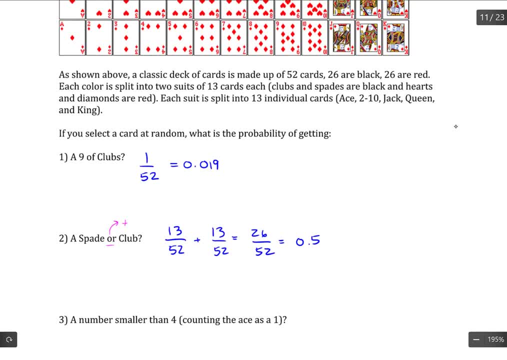 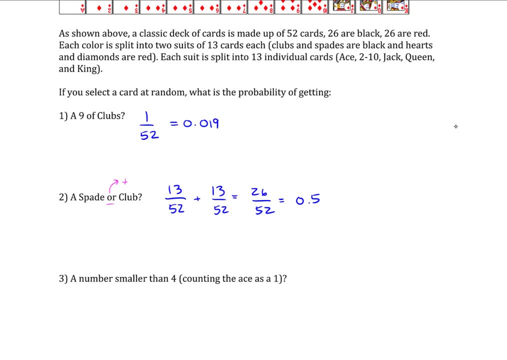 fourth plus one. fourth would also give us one half, A number smaller than four, counting the ace as a one. So sometimes the number is smaller than one and sometimes the number is smaller than one. Sometimes the ace is counted as a one, sometimes it's counted as higher than a king. 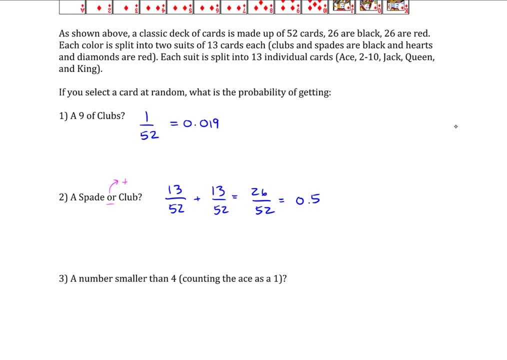 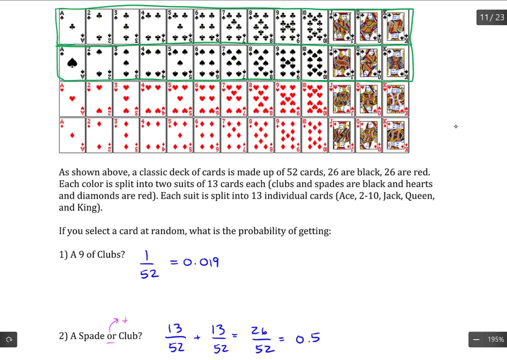 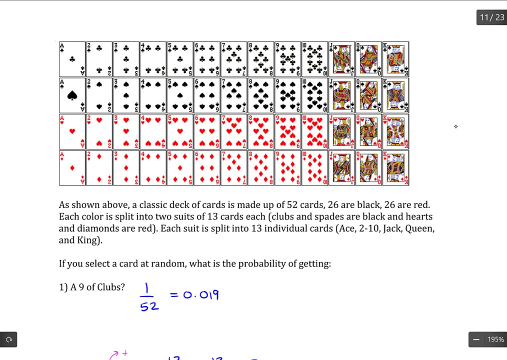 sometimes it's not counted as anything, it just depends. In this particular case it's defined as a one, So we want the probability of a number smaller than four. So a number smaller than four, the ones that qualify here are ace through three, But it could be in any of the suits. 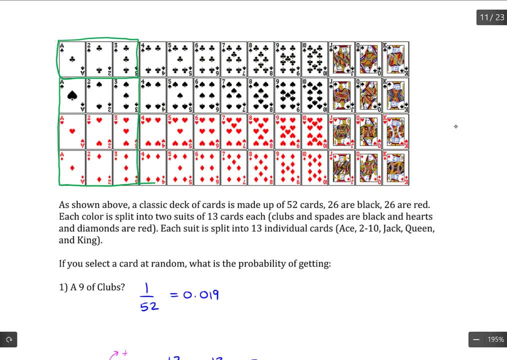 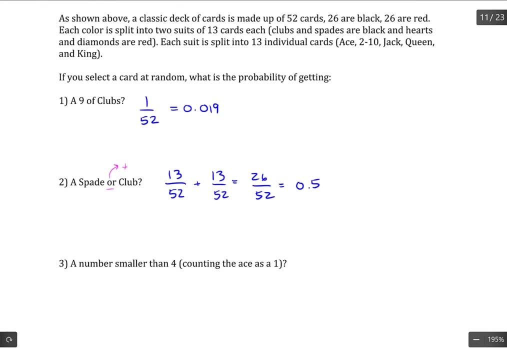 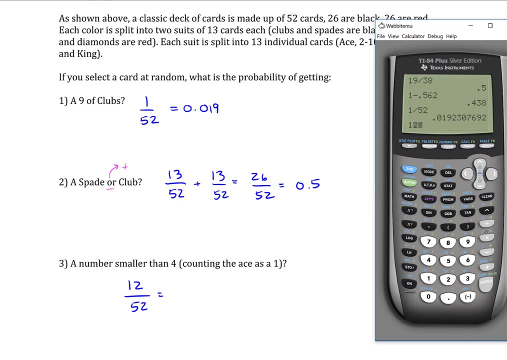 so it could actually be in any of the suits. So we want the probability of a number smaller than four. So that gives me three cards out of each suit by the four suits. So that means my probability is 12 over 52.. 12 over 52 gives me 0.231.